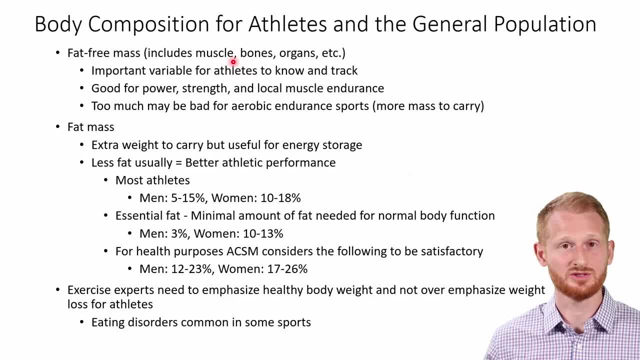 little bit of bone, but mostly greater muscle mass. So athletes tend to want to increase their fat-free mass because it's good for most athletic events- not all, but most- So it's going to be really really good, obviously, for power and strength. 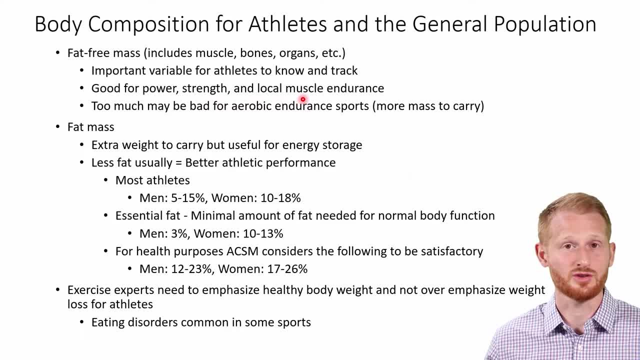 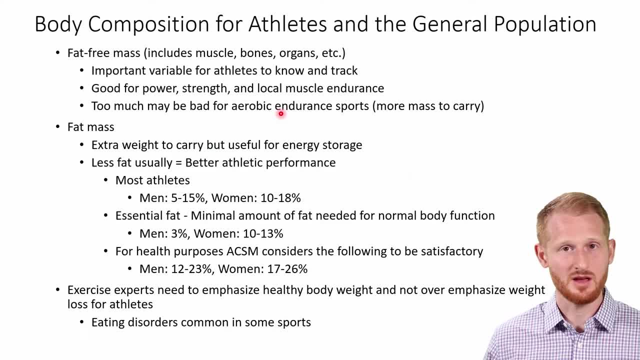 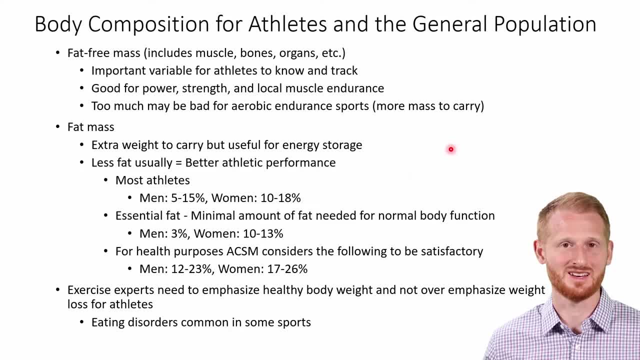 Some muscle mass is still good for those athletes, but maybe an excessive amount of muscle mass is not going to be helpful, might actually hinder those sports. But for the most part, most athletes want to increase their lean muscle mass. Fat mass, on the other hand, is 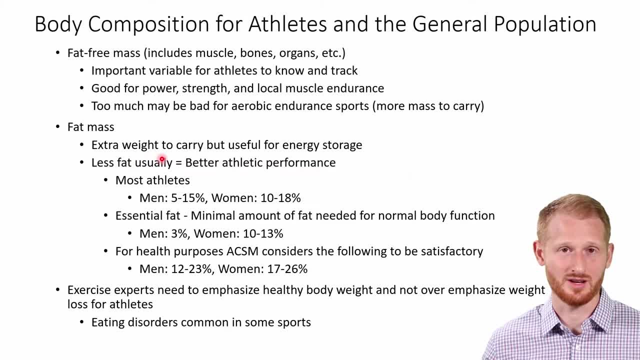 something that is extra weight to carry during an athletic event. So most athletes want to decrease their fat mass to a healthy level, but decrease it lower than what the average population tends to have. Fat mass is good for some things, mostly for energy storage. There's a lot of 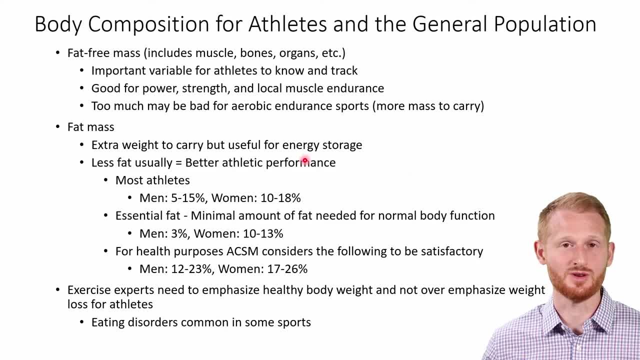 ATP that can be liberated, which is our energy unit in our body. So there's a lot of energy in fat that can be liberated and used during athleticism or exercise, And so we do need fat in our bodies in order to do that. 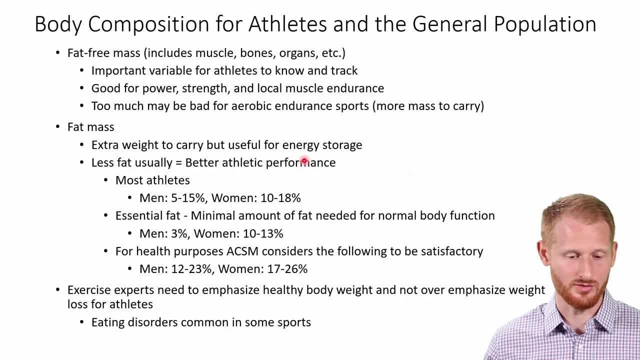 both for athletic reasons as well as health reasons. But generally speaking, less fat usually means better athletic performance. Again to a point. Most athletes, for men are going to be between 5 and 15 percent body fat. For women they're going to be between 10 and 18 percent body fat. 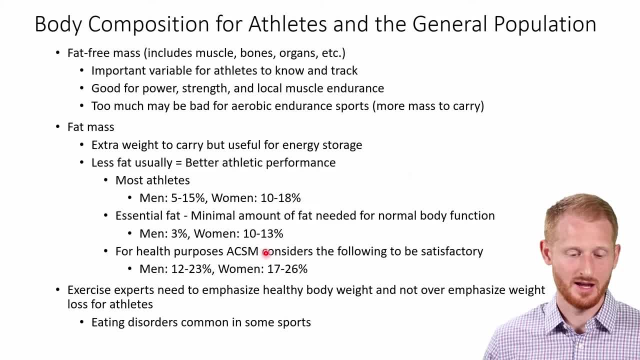 So this is sort of just generic feet profiles. Keep in mind, as I've already alluded to, you do need body fat and you don't want to be too low with body fat because you can start running into various issues with your health as well as with exercise performance. So there's a term called essential fat, which basically means 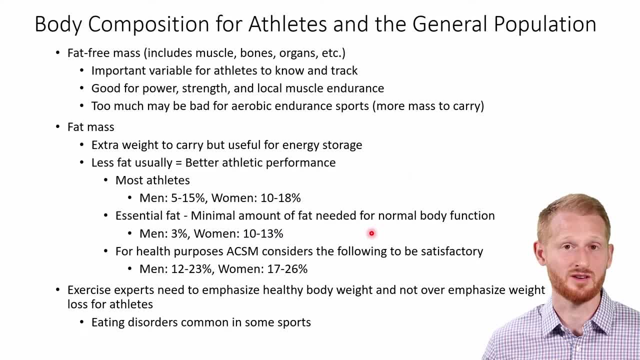 the minimal amount of fat the person can have with having normal bodily functions. Now, this does vary by person, so not everybody can get as low as the values on this screen. but the these are the values from the ACSM's primary textbook, their guidelines textbook. So for men, 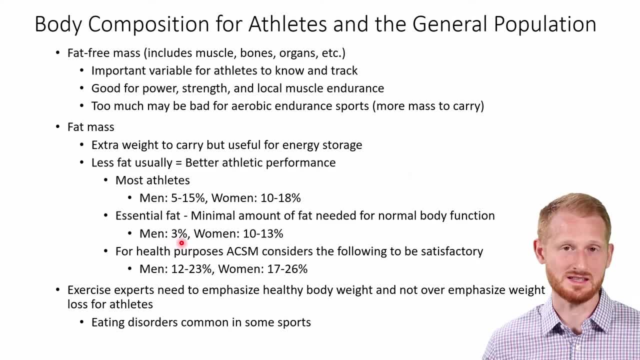 below 3 percent body fat, you're likely going to start seeing some health and physiological issues. For women below 10 to 13 percent, It's a little bit of range there again, because not everybody's the same and there's some discrepancy in the data out there. So 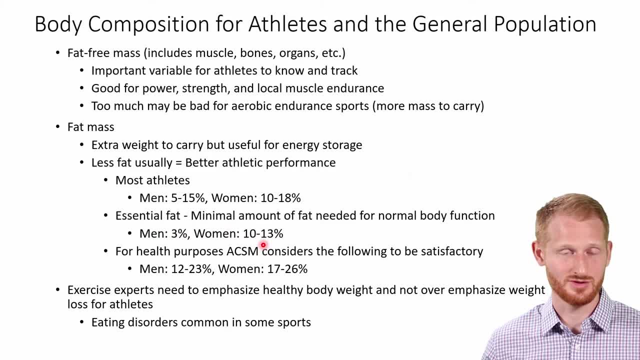 below these essential fat levels, you should definitely expect to see some negative health consequences. For some people, there are negative health consequences above these levels. This is actually something we're getting much more aware of in the exercise research community. Things like the female athlete triad and also now the male athlete triad that they're 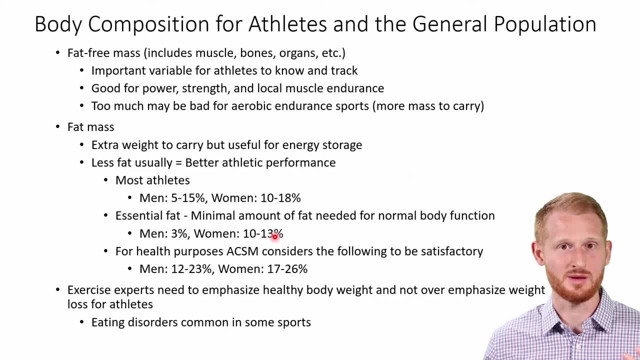 starting to recognize in research as well, is when people have consistently low body fats and it can lead to some issues with hormonal balances and bone density and various things like that. But in sticking to just what is in the sort of ACSM guidelines right now, don't go below 13,. 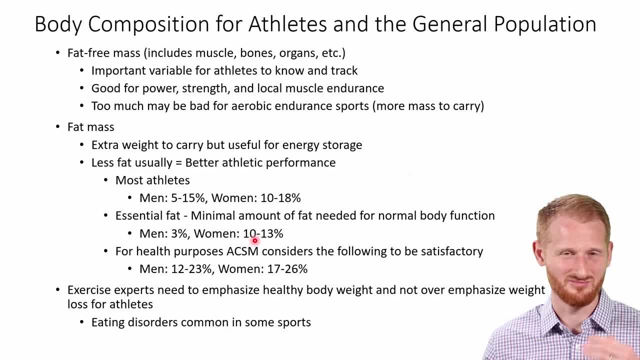 or 3 percent for men, 10 to 13 percent for women, Being a little bit above, that's probably a good thing, All right, so for health purposes though. so this is not talking about athleticism at this point, just sort of a general population. the ACSM considers it satisfactory for men to be between: 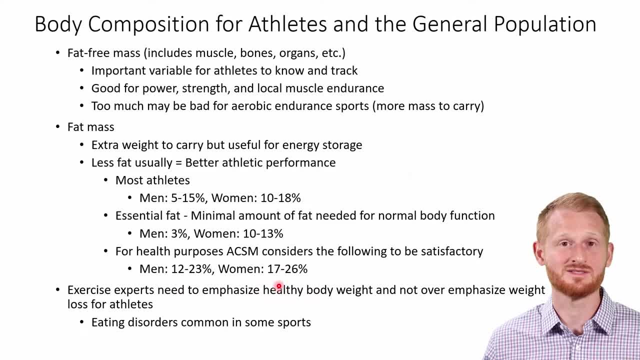 12 and 23 percent body fat and for women to be between 17 and 26 percent body fat. And I say the satisfactory with the the quotes, because there is not a standard that everybody agrees to about what is considered good body fat percentage. This is the reason why we don't 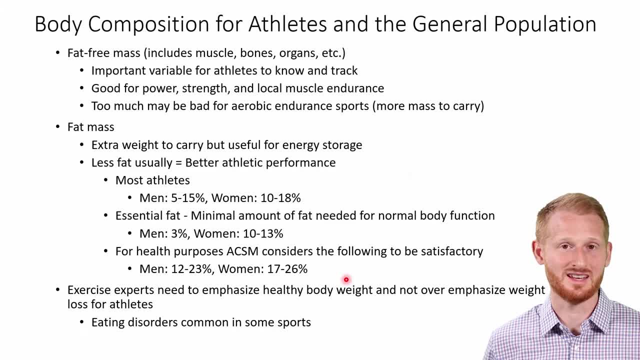 generally use body fat percentage in order to identify if somebody is considered obese or overweight. We more use it as a way of determining what their percentile rank is, or categorical rank specific to the percentile rank for body fat. Again, we've already talked about this in our previous video, but we don't typically use this to 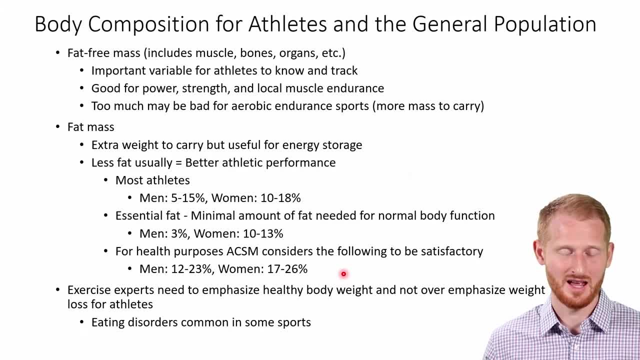 determine if someone's overweight or obese. We would use body mass index, or BMI, more commonly to do that. I already have a video talking about the basic anthropometric measurements, so I'll put a link in the description below this to that video. As exercise professionals, 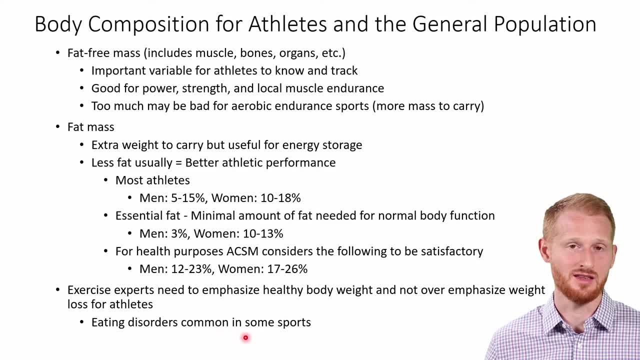 we need to be looking out for signs of eating disorders. It's very common in some sports for people to have eating disorders. especially the sports tends to lead to greater exercise performance. So think long distance running, cycling, all the aesthetic type activities in sports, Think cheerleading gymnastics. They oftentimes 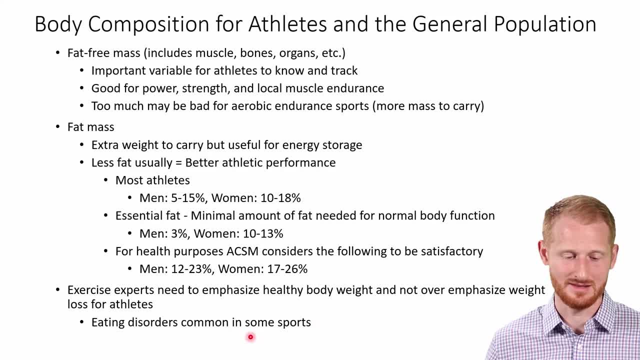 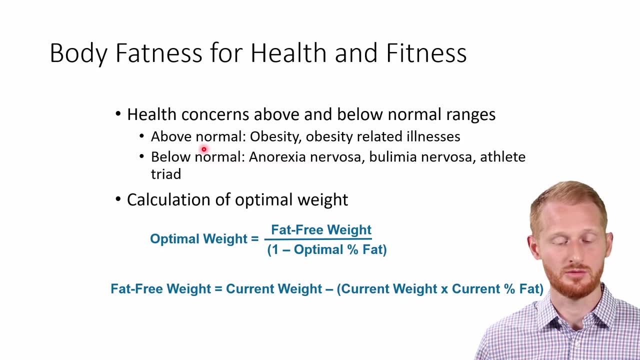 will have very low body fat percentages and sometimes that can be driven by disordered eating. So again, if you're working with those athletes, it's something to be aware of. There are concerns with having a very high or very low body fat percentage, So above normal body fat percentages. 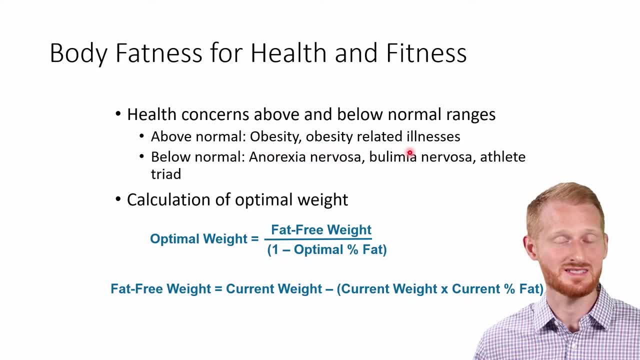 means a greater likelihood of obesity or obesity-related illnesses. So things like cardiovascular disease, diabetes and several others. Being below normal, so being sort of under fat, leads to a greater likelihood that the person might have some sort of eating disorder like anorexia nervosa or bulimia nervosa. It also increases the likelihood 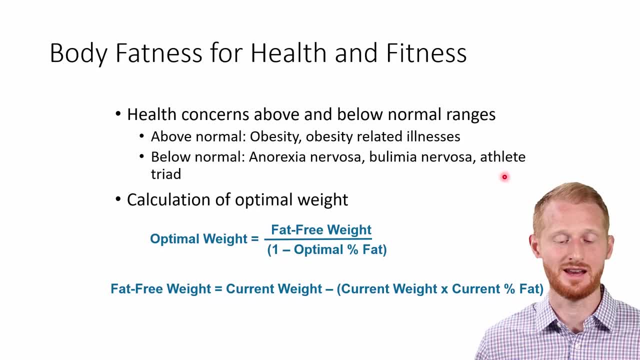 that they might have some sort of eating disorder. So, again, if you're looking for some sort of eating disorder, you might want to look at the athlete triad, So both the male and female athlete triad, And so those are all very serious conditions as well that you would want to avoid, And there are, 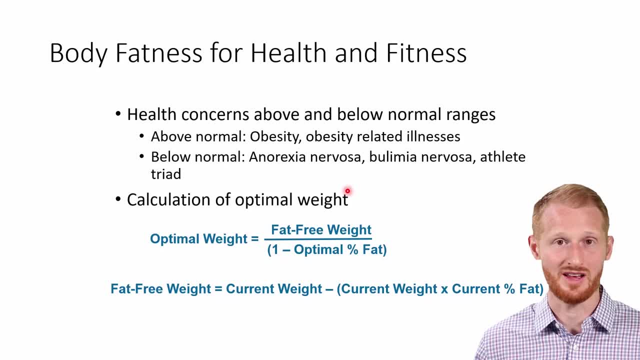 other ones as well that are associated with low body fat percentage. that could cause some issues for their health. This is just sort of ones to look out for. With that in mind, you need to be able to determine what the optimal weight of the person would be If they were to achieve the body. 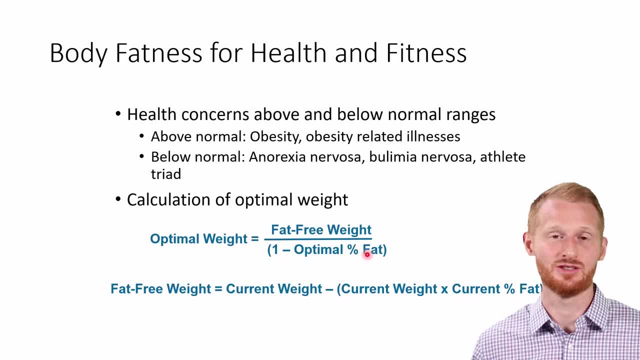 fat percentage that they're looking for And that body fat percentage should be something they look up in some sort of normative chart based typically around the good categories- Good to maybe excellent categories- where you want to be for most people, both for health and fitness reasons.